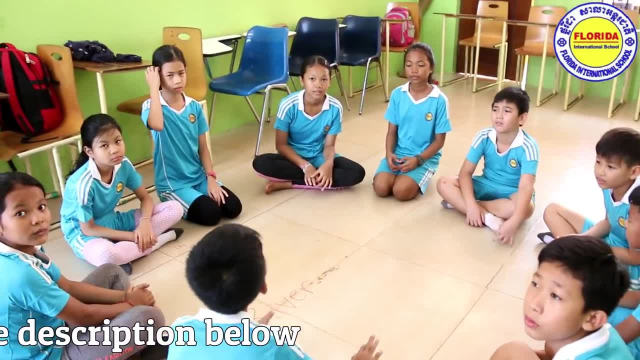 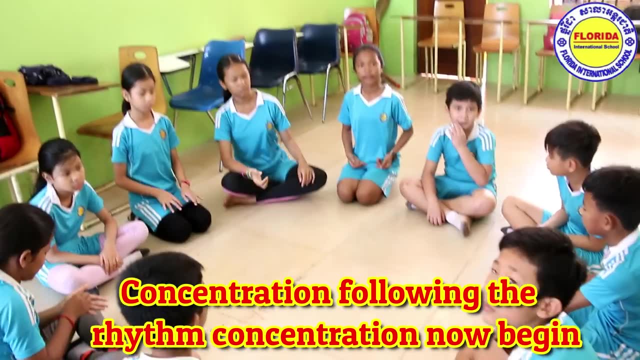 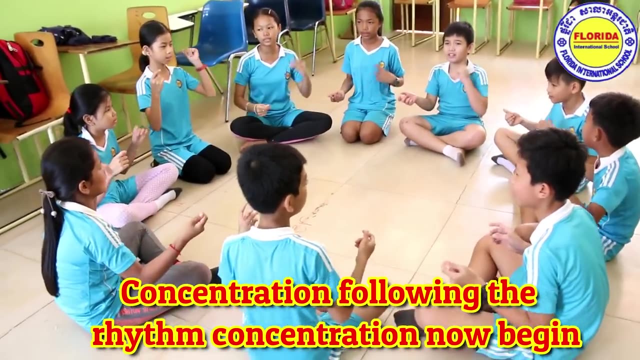 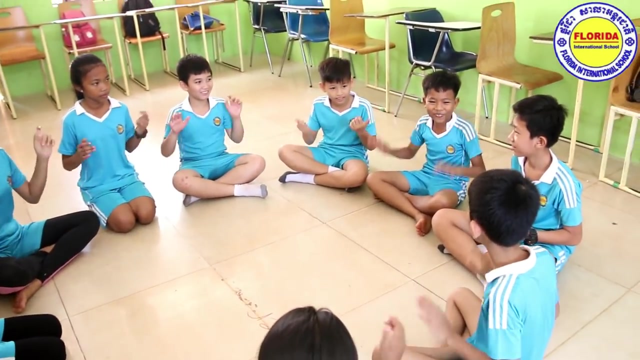 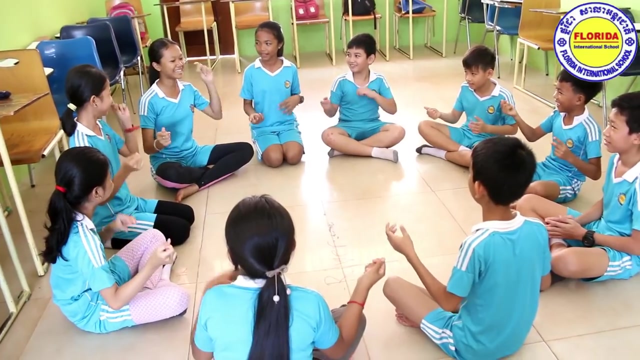 It's over ten. You're going to say your number first and then you pass it to the other student. So let's practice. first Concentration: Ready, Go Concentration. Following the Rhythm. Concentration. Now begin: One, two, three, four, five, six, seven, eight, nine, ten. 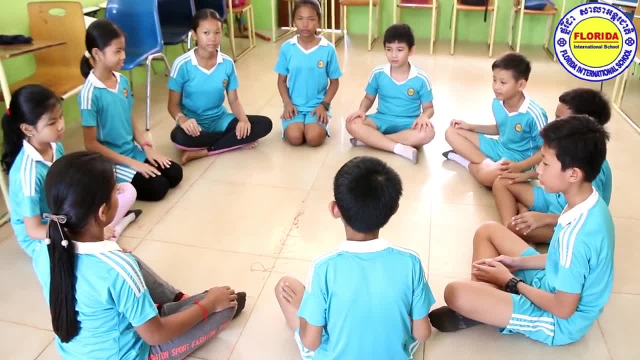 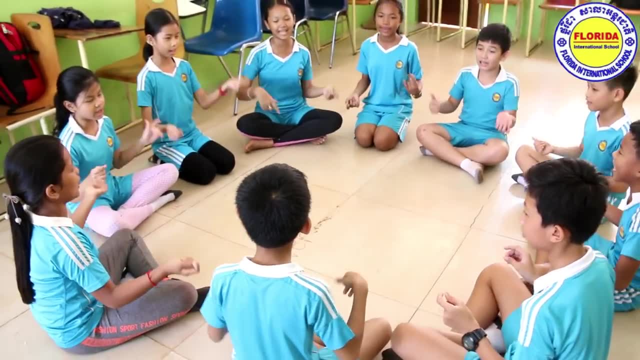 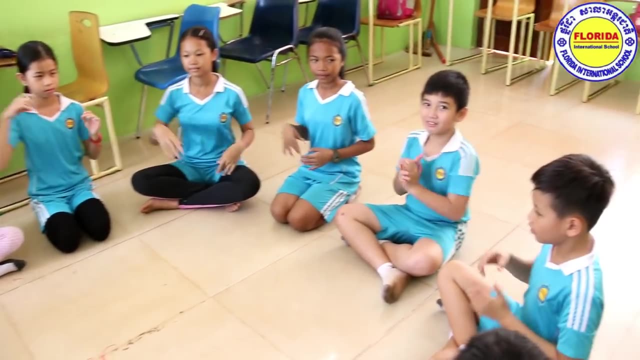 Let's start now. Let's start with number five. Number five Ready Start Concentration Following the Rhythm. Concentration Now begin: One, two, three, four, five, six, seven, eight, nine, ten. 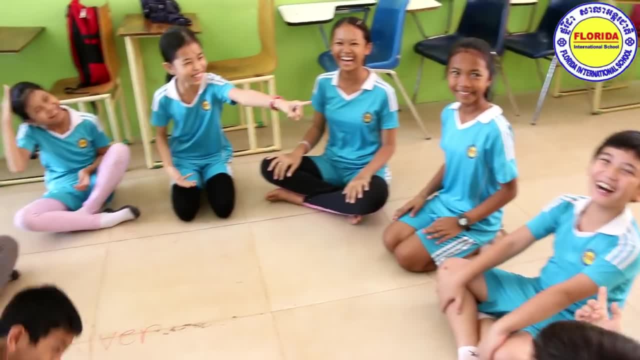 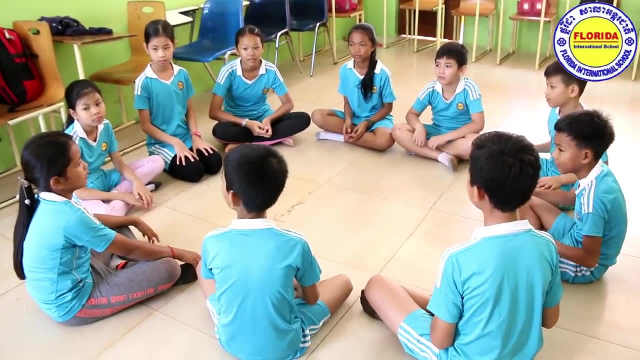 It's over ten. You're going to say your number first and then you pass it to the other student. You're going to say your number first and then you pass it to the other student. Number five. Okay, Let's start from number six. 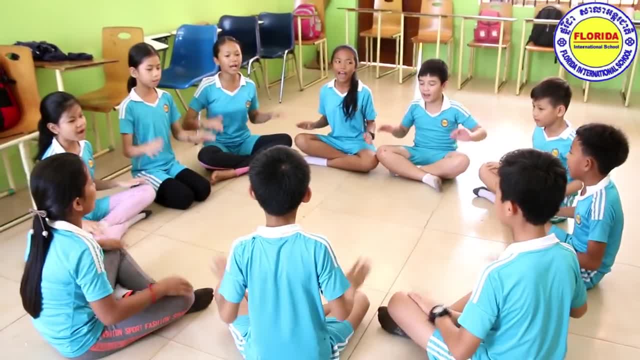 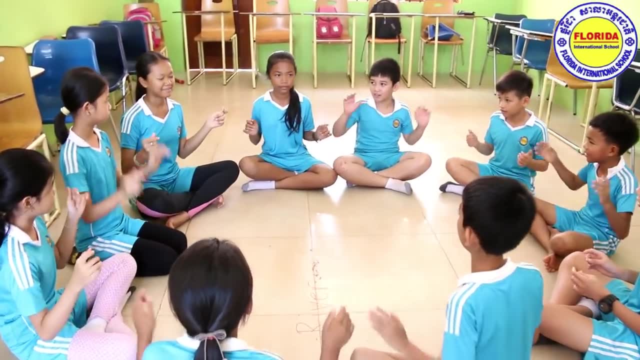 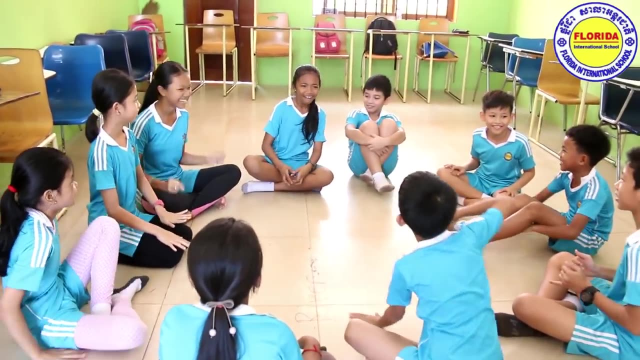 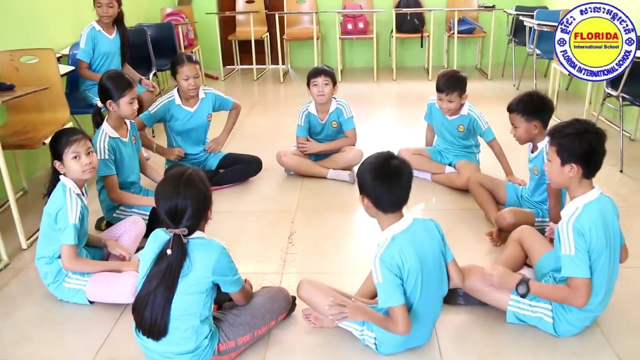 Ready. Start Concentration. Following the Rhythm. Concentration Now begin One, two, three, four, five, six, seven, eight, nine, ten out. Okay, ten is out of the group now, so let's start with number three. 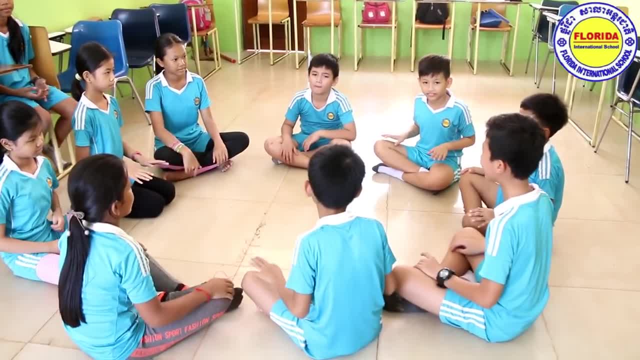 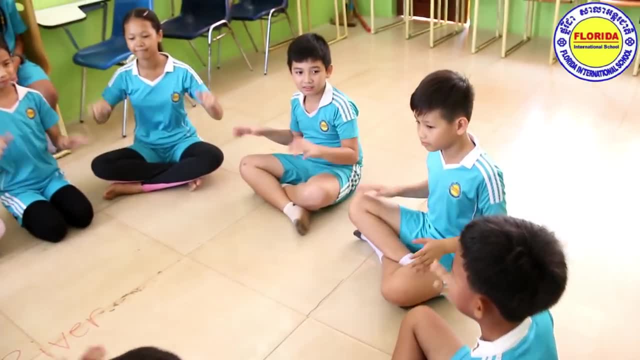 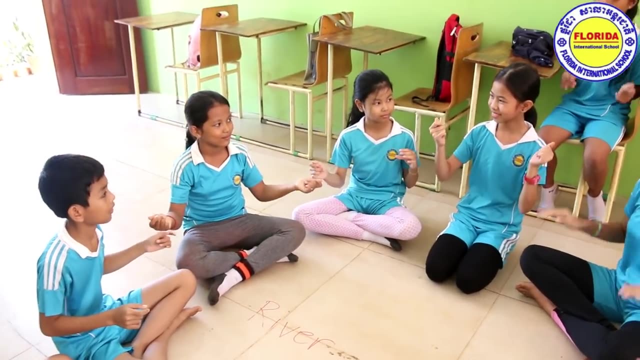 Three Ready Start Concentration Following the Rhythm. Concentration Now begin: 1, 2, 3, 4, now we get it: 3, 2, 2, 6, 6, 8. Okay, let's start with the last one. 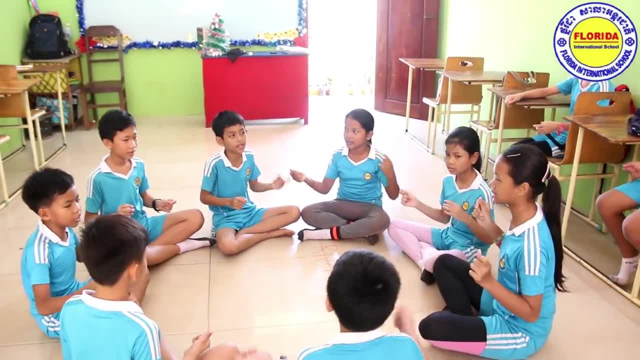 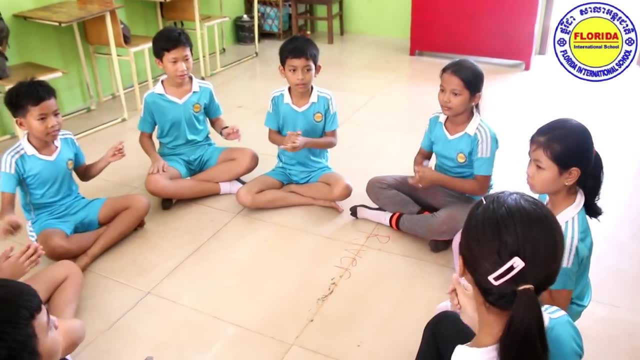 Ready. Start: 1,, 2,, 3,, 4,. follow with the rhythm: 1,, 2,, 3,, 4,. now we get it: 6,, 7, 7, 8, 9, 10. 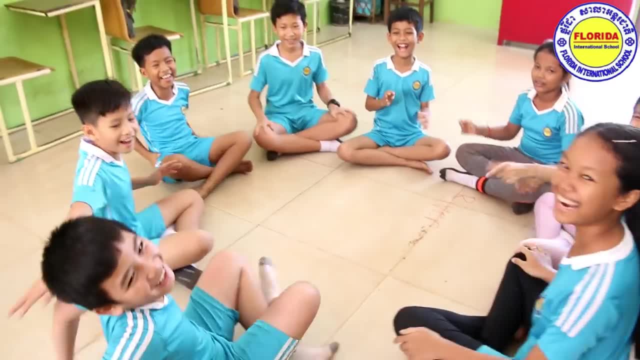 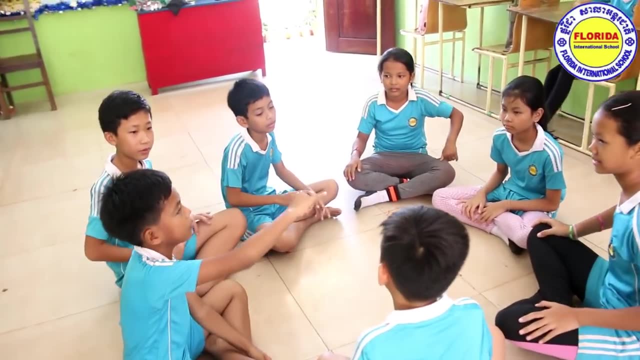 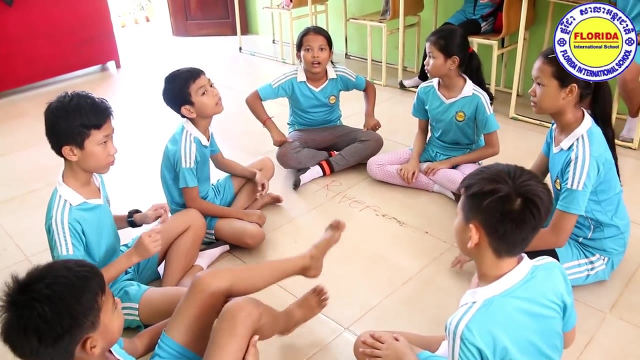 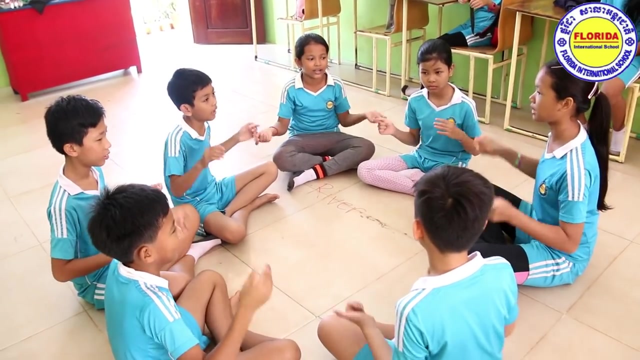 1, 10. Okay, remember those numbers who are out already: 1,, 2,, 3,, 4,. follow with the rhythm. Ready, Let's start again from Who's the last? Okay, ready, Start. 1,, 2,, 3,, 4,. follow with the rhythm.